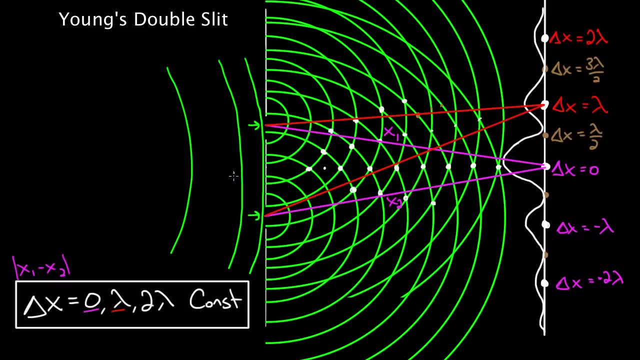 Okay, so that's all well and good, but we've got a problem. I told you, these two slits are so close together, maybe micrometers or nanometers. apart that, how are we going to measure? How are we ever going to physically measure the difference in path length? 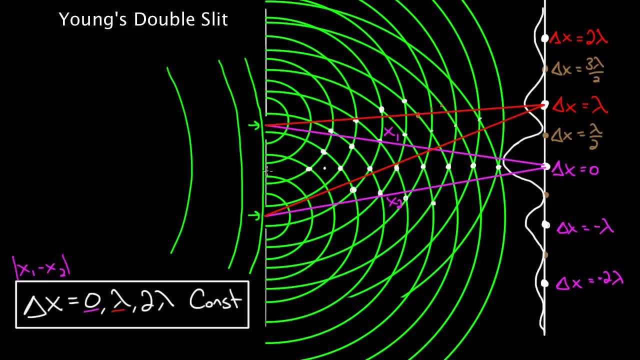 If I go over to this barrier, these two holes are going to look like they're at the exact same spot. That's how close they are. So I need some way to determine the path length difference based on something I could measure, And that's where we're going to have to play a trick here. 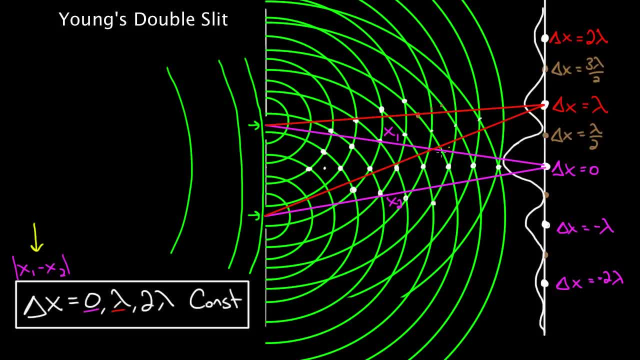 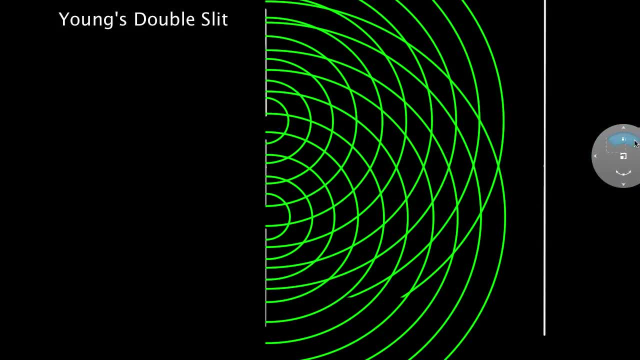 We're going to have to figure out a function for this path length difference based on what angle I'm at. So the basic idea is this. So let me get rid of all this And let me put it to you this way. So let's say, I draw a reference line. 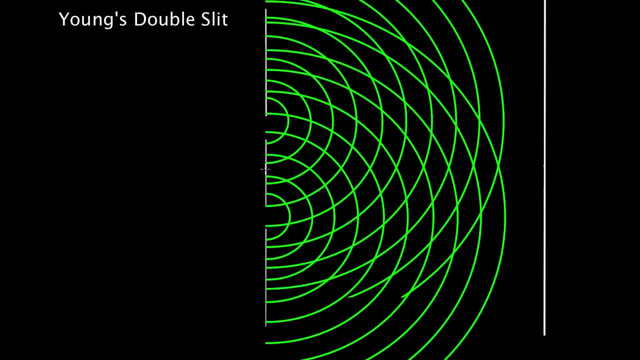 A reference line that goes straight through the center. This center line is my friend. This is going to let me measure angles here. So we've got this line here. Let's say I wanted to measure to some point on the wall. What angle am I at? 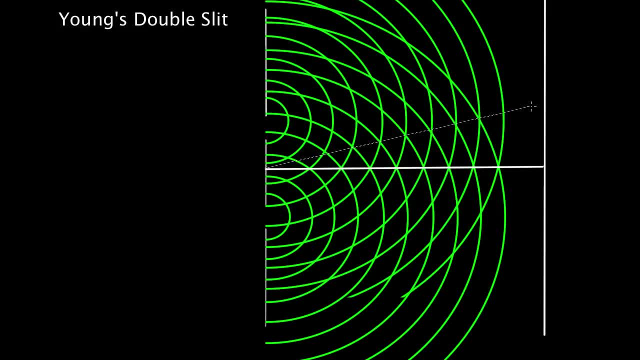 This is how I'm going to measure the angle From this center line to some point over here. let's say Like that, So my angle is going to be this. So this here would be my angle And my question that I'm asking is based on this angle. is there some way to determine the path length difference? 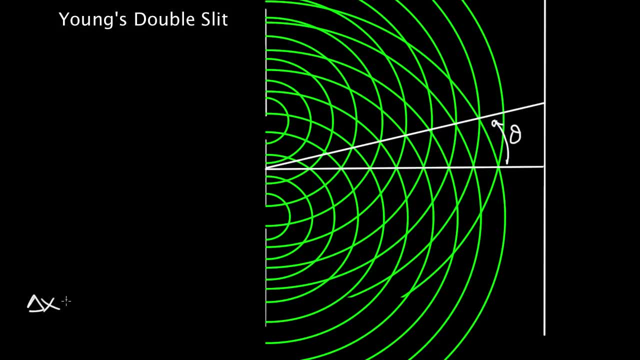 That's the important thing here: How do I determine the path length difference? How is the path length difference related to this angle? The way we can do it is this: If this screen is far away, here's what I'm going to do. 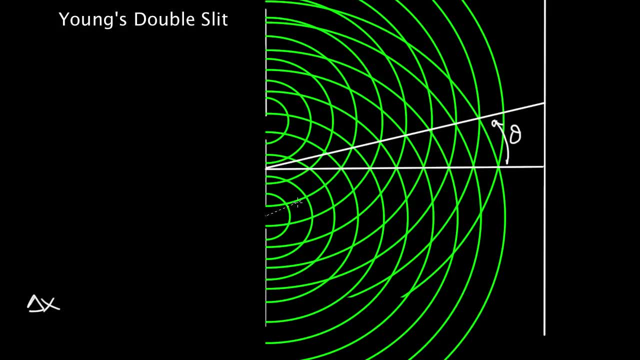 I'm going to draw a line from the center of this, This bottom slit, to that point, And I'm going to draw a line from the center of this top slit to that point. And if this screen is far away, significantly further away than these two holes are spaced, 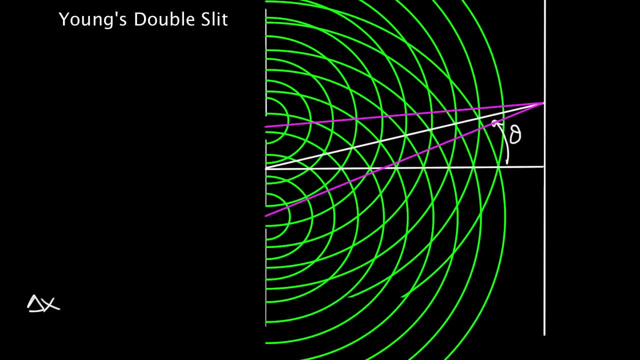 which isn't too much of a problem because these holes are very close together. I can draw a third line and this third line is going to look like: this Third line is going to go from here down. cut through this at a right angle. 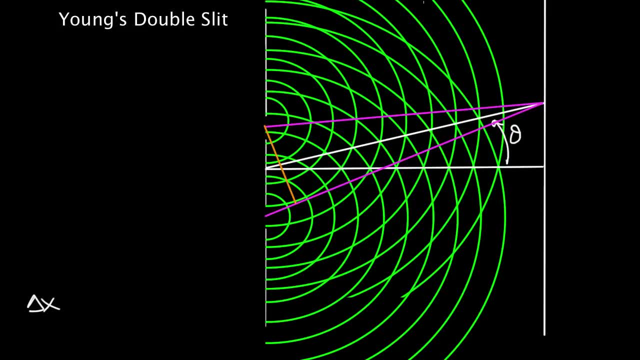 And if I'm far away, if my screen is far away, what will be true is that if this is a right angle right here, then the remainder of these paths will be equal. In other words, the path from here onward, from here forwards, will be the same length. 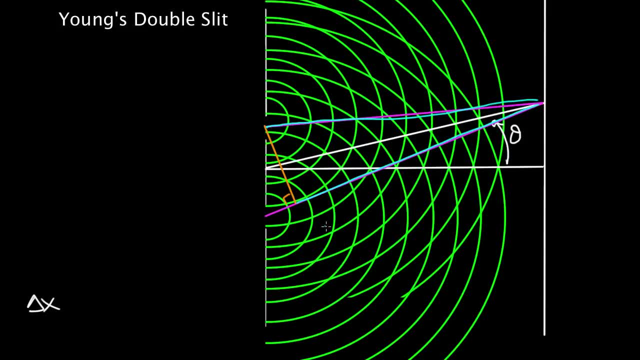 as the path from here forwards. So what would the path length be? The path length difference would just be this piece down here, whatever's left. This would be the path length difference. This is delta x, in other words. So how do I find this? 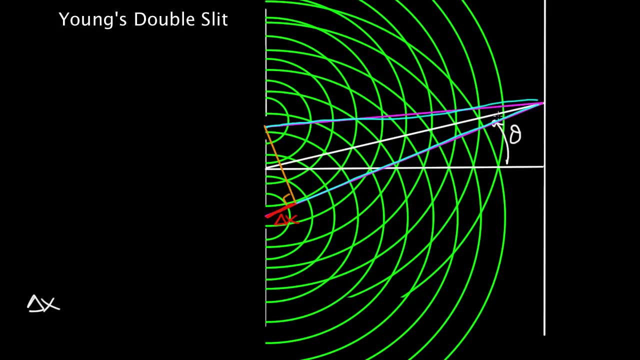 Well, again, if I'm far away here, This angle here will equal this angle inside of here, So these two angles are the same. So now that I know that these two angles are the same, it's just basic trigonometry. 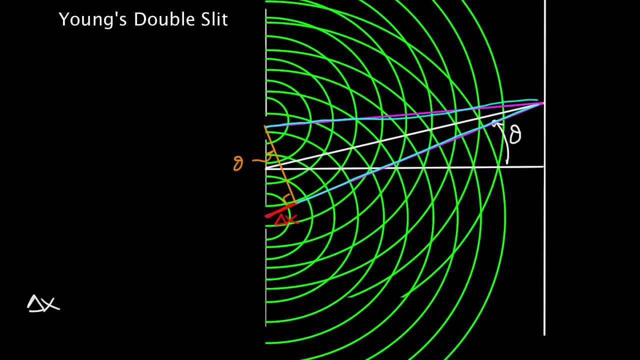 I've got a right triangle in here and I'm going to redraw it over here. I'll just draw you a right triangle. So my right triangle looks like this: I've got this distance between the holes, which is D. I'm going to call that distance D. 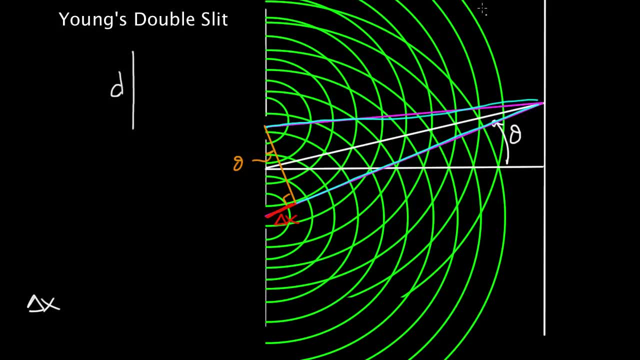 The distance between the two holes, Center to center distance. And then I've got this up, This other orange line. This represents that line I had to draw to make the right angle. And then I've got this path length difference this way: 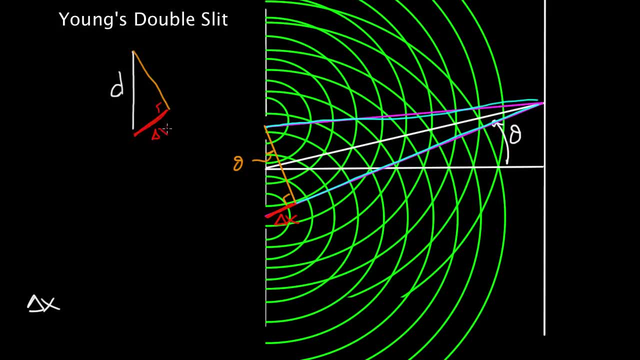 So this is my triangle and this is supposed to be a right angle. This side's delta x, The path length difference, The extra amount that wave from the bottom hole had to travel compared to the wave from the top hole. Well, this is trigonometry. 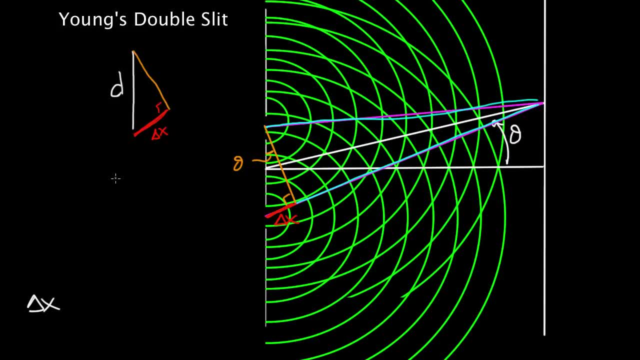 Here's my right angle. I can just say, if I want a relationship between these, I can say that sine of theta, Because this is theta And that theta is the same as this theta. over here, Sine of theta would be opposite over hypotenuse. 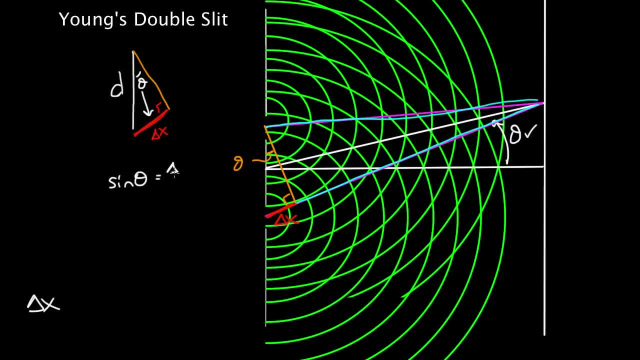 And the opposite to this theta is delta x. So I have delta x over the hypotenuse. in this case is D This entire distance between the two holes, Because this side's the right angle. The hypotenuse never touches the right angle side. 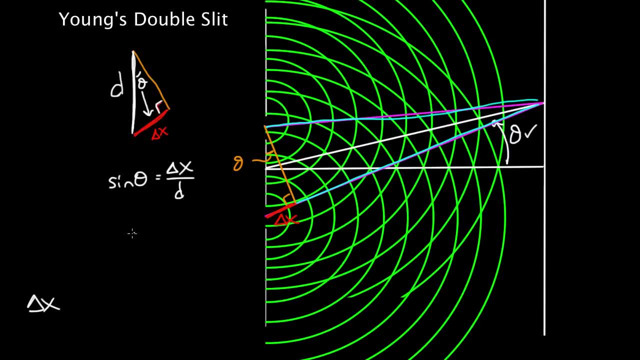 The hypotenuse is this other side, So that's over D. So what's the path length difference D? The path length difference for a double slit is just D times sine of theta. So this is what I wanted. Now I know delta x is D sine theta. 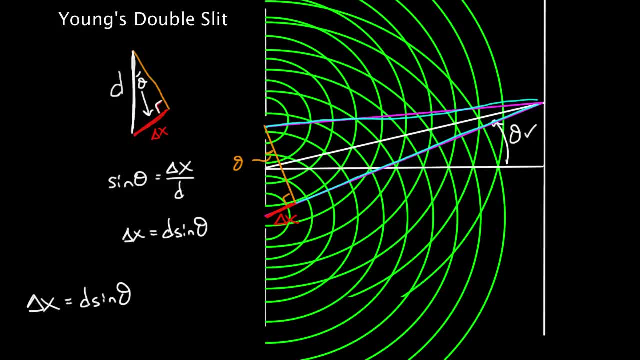 And I can write. Now I can write the double slit formula. Let me get rid of this. The double slit formula looks like this: It says that M times lambda equals D sine theta. And why? Well, remember Delta x for constructive points. 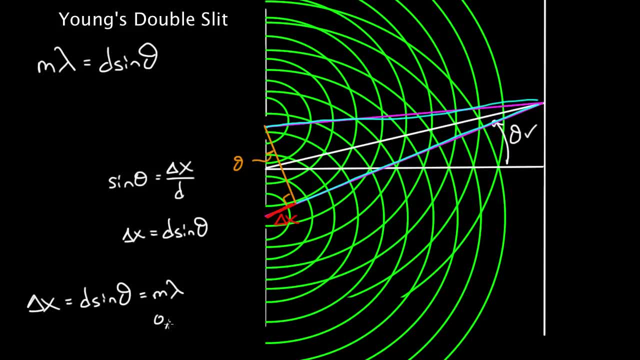 Was integers, times wavelength, So zero: one wavelength, two wavelength, and so on. And so, in order to get constructive points, D sine theta, which is the path length difference, has to equal zero lambda, two lambda, And this is the double slit formula. 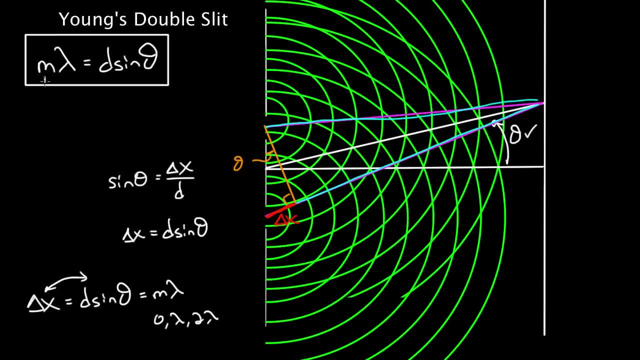 It looks like this. What does it give you? This M is going to be zero, one, two and so on. The D is the distance between the two slits. That would be D. Theta is the angle from the center line up to the point on the wall where. 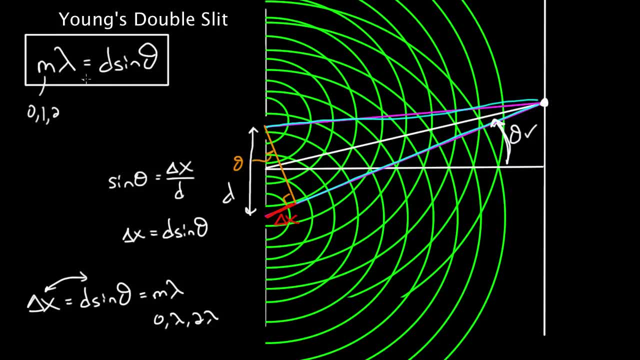 you have a constructive point, And lambda is the wavelength. Lambda is the wavelength, The distance between peaks of the wave. Now, I mean theoretically speaking. you could plug in one halves for M And that would give you the angles to the destructive points. 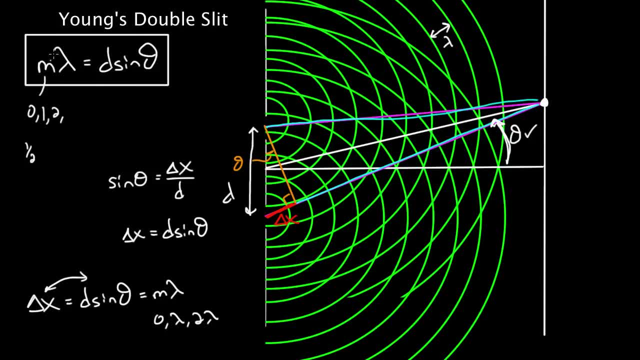 Because we know that delta x, the path length difference, should just equal half lambdas to get to the destructive. So this can give you Angles to constructive points and destructive points if you plug in the correct M value, the order. Sometimes this is called the order of the constructive point. 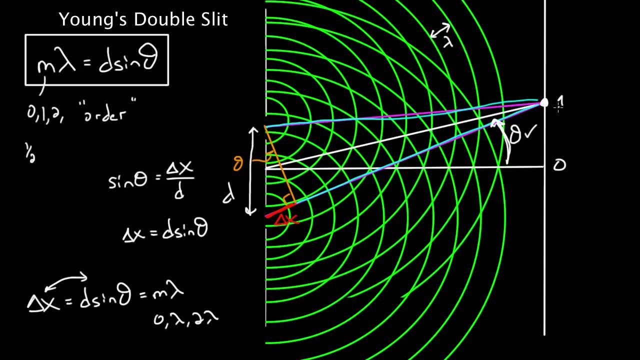 This would be the zeroth order, because path length difference is zero. Sometimes this is called the first order because it's one wavelength difference. The next one might be called the second order because it's two wavelength difference. You might object, though. 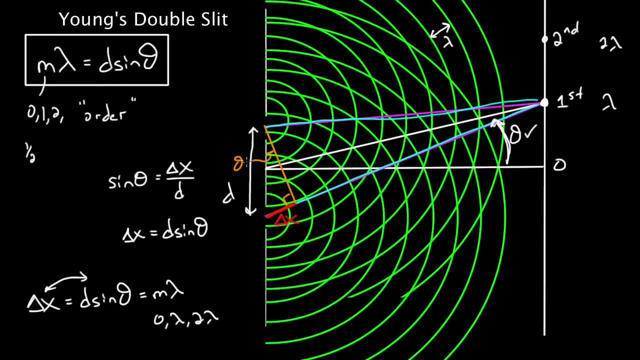 You might still say: wait, this was no better because D is really close together. The D spacing right here is extremely close. We can't measure that well, but we can measure theta And we can know that wavelength of the laser we send in.